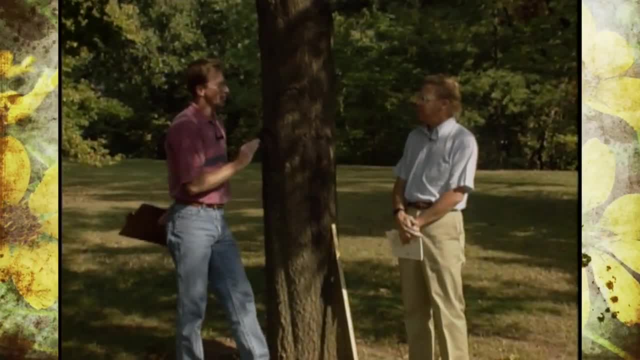 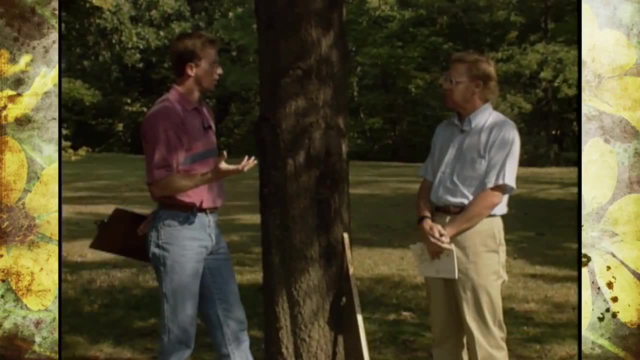 And Bob, welcome to Oklahoma Gardening, Thank you. Now, Bob, you're going to tell us about how we can come up with the value of a tree and tell us a little bit about why people maybe need such numbers. To begin with, what are? 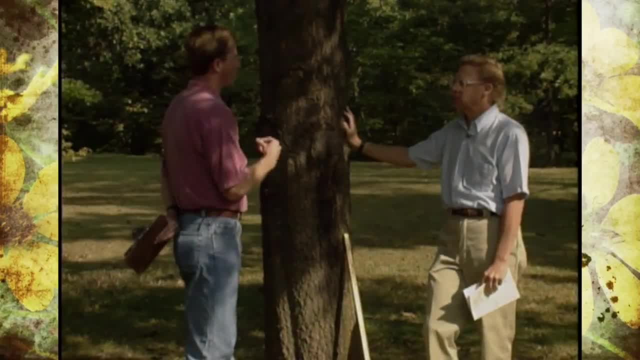 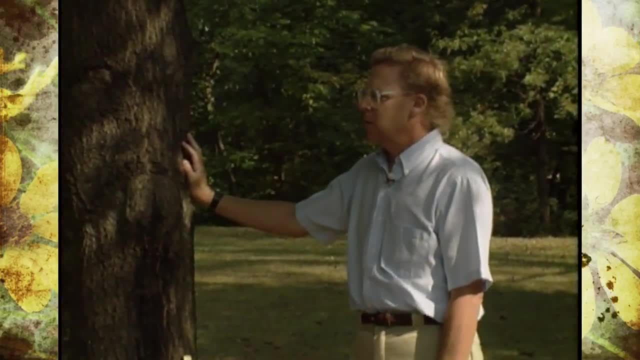 some examples in your experience why people would need the value of a tree. I understand in visiting with you there are several different reasons, maybe from accident fire. Why don't you elaborate on that for us? Well, trees can be damaged in many different. ways. Naturally, trees can be damaged in storms, tornadoes, ice storms, and there may be a need to value the tree for insurance or casualty Casualty loss reasons. Trees can be damaged, particularly in urban areas, by vandalism or accidents, For example, an automobile losing control and leaving the road and running into. 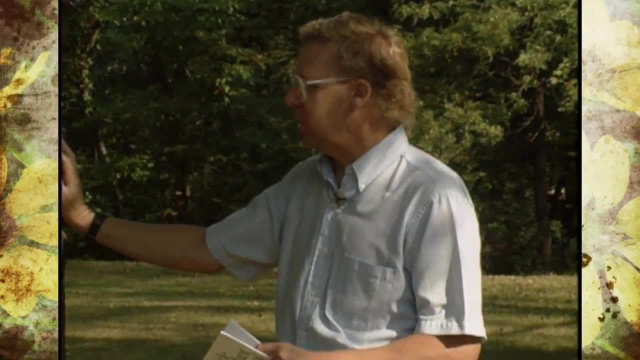 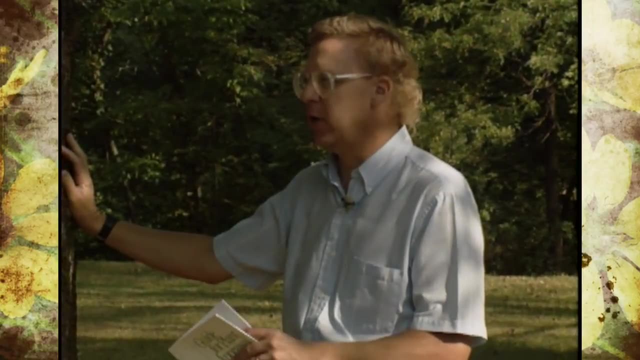 a tree, damaging the tree. Sometimes trees are damaged as a result of negligence on the part of others- Starting a fire, for example, and having it spread off of their property onto somebody else's property, and burning trees Leaks in pipelines. 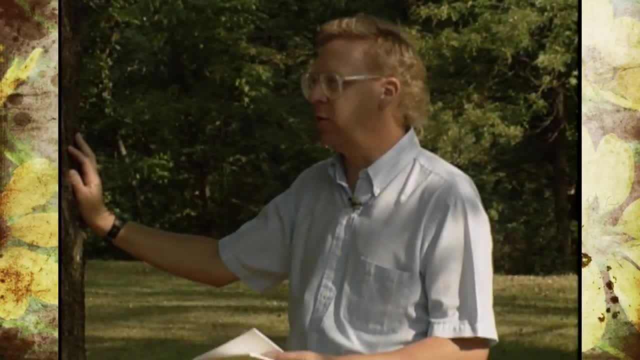 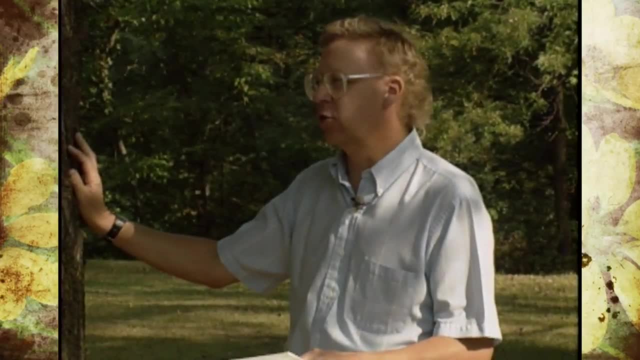 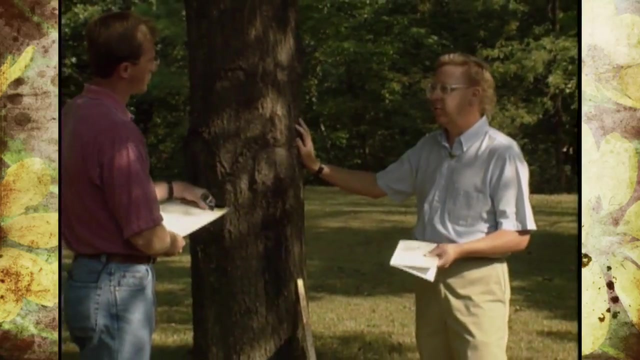 For example, can cause damages to trees, or the cleaning up of those contaminations can lead to the damage of trees. So there are really lots of different ways in which trees might be damaged and in order for the person who owns the tree to be compensated for that, 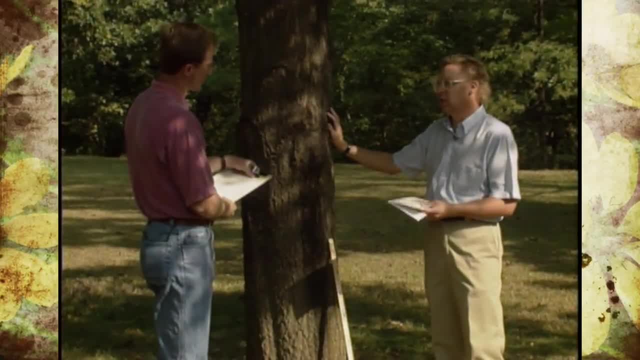 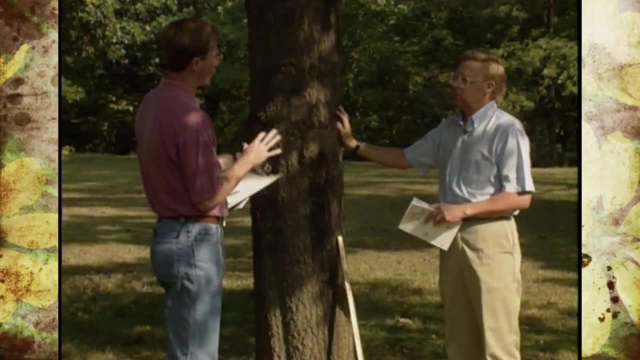 loss, then we need to determine what the value of the tree is to come up with a fair settlement. Okay, Now there's also many ways to determine that value too- Several methods. Why don't you tell us a little bit about the value of the tree? Well, the value of the tree is a. 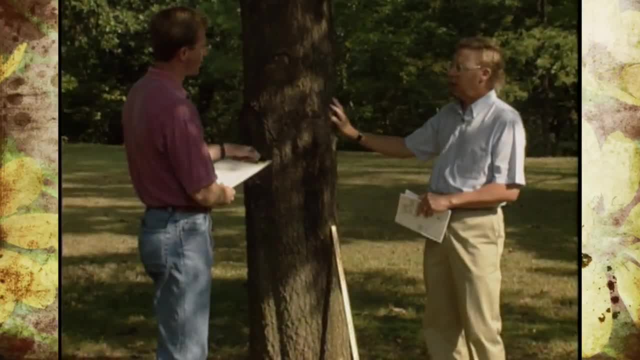 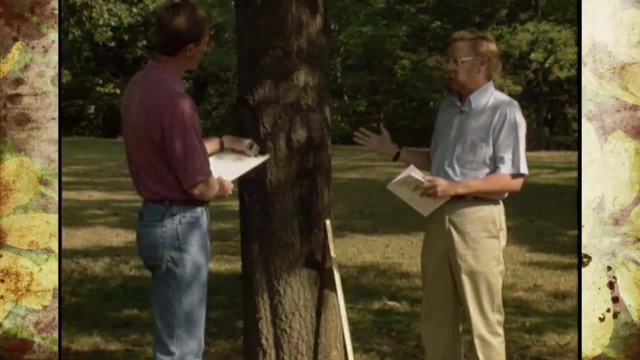 lot of different things. You can tell us about some of the methods, and then we might go into some details. Okay, The first thing that I look at when trying to determine the value of the tree is: what was the use of the tree, As you probably are aware, here in Oklahoma, 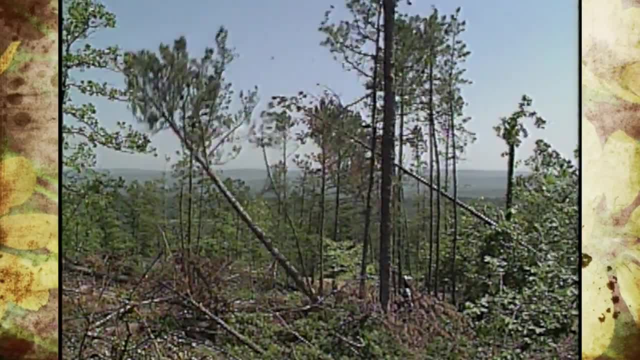 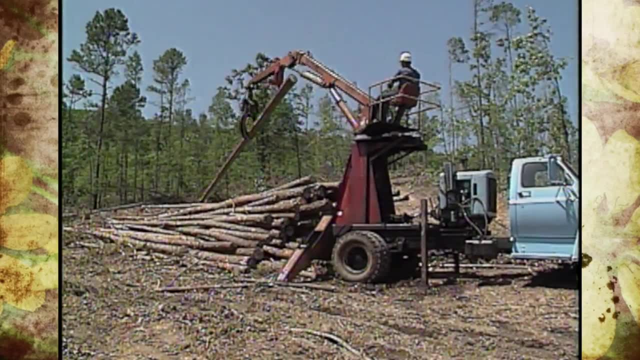 in the eastern part of the state we have a lot of commercial timberland. If the trees that were damaged were being grown for the intent of making paper or timber products, then we would use whatever the market value is for that type of commodity to determine. 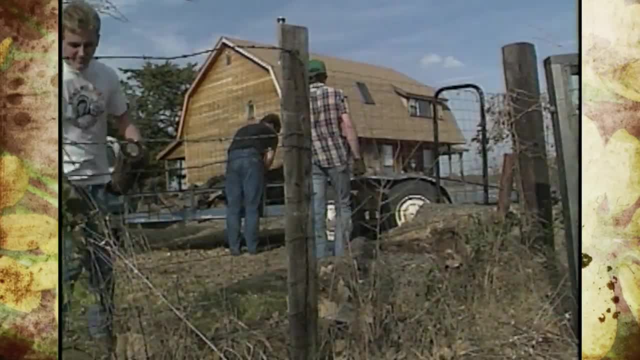 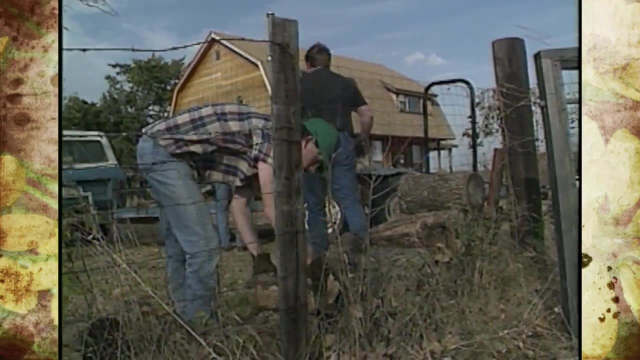 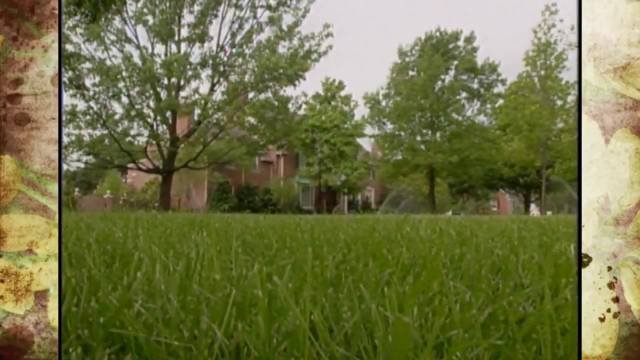 the value of the trees. Some people cut trees down for firewood production and if those trees were damaged or lost, then we could determine the volume of firewood that would be available from those trees and figure out a value in that respect In many cases, most. trees don't have a particular commercial value and therefore we have to come up with a different method to determine the value of the tree, and there are some formulas that have been utilized for a number of years to help determine the value of non-commercial trees, And that's. 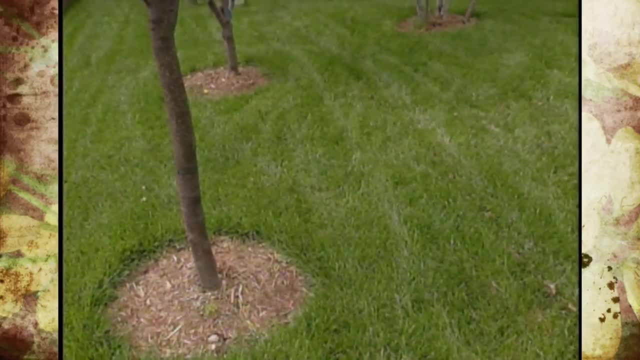 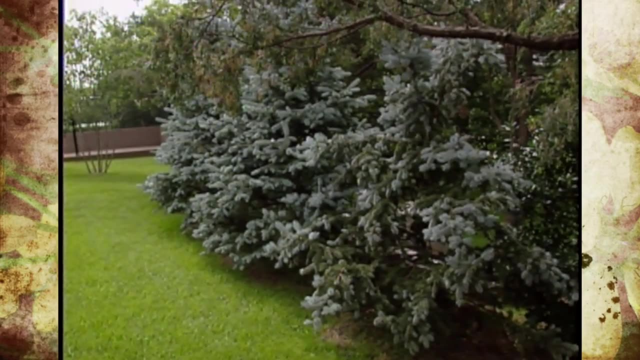 probably what we would use more in a home type situation in many cases. Now, if it's a smaller tree, say one we've just purchased, and the caliper is pretty small, there's a different method for that compared to a large shade tree. Is that true? Yes, If the tree is available in a nursery. and when I say if it's available, a tree of the same type and the same size, Then the loss would be what it would cost you to go and purchase that tree, generally retail price plus the cost of having somebody plant the tree for you and maintain that tree. normally for a year, sometimes even two years, and also the cost of cleaning up the debris that would be left behind when the tree is, when the original tree has been damaged. So all of those costs combined would be the loss to the property owner if a smaller tree is. 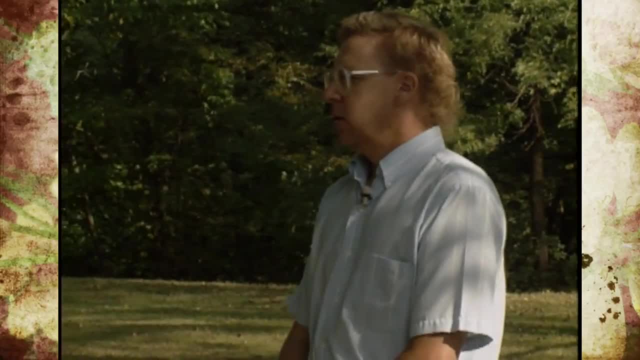 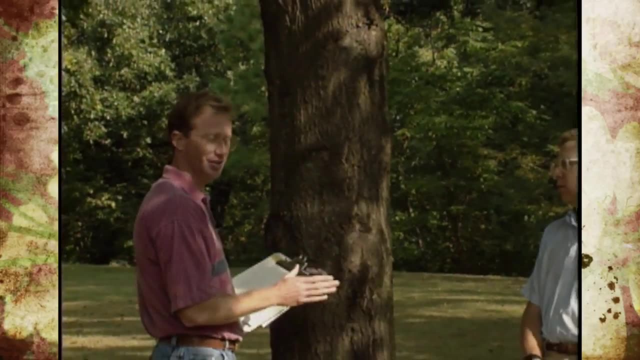 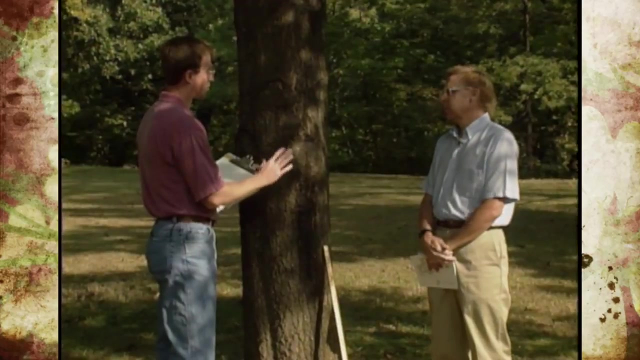 damaged. Okay, good. Now, in a case like this with a large tree, we're looking at a little bit different situation. I understand, Bob, that the formula has just recently changed. what this year, as a matter of fact, Right? First of all, who comes up with these formulas for appraisals? Tell us a little bit about. 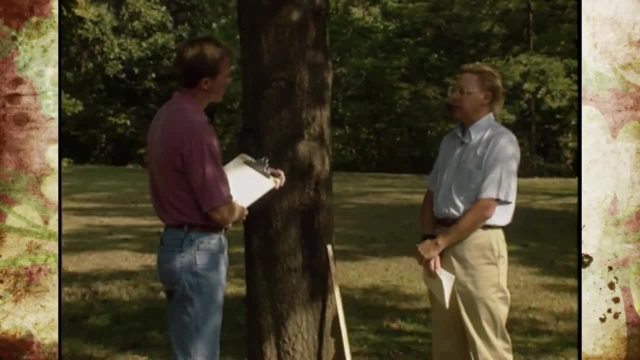 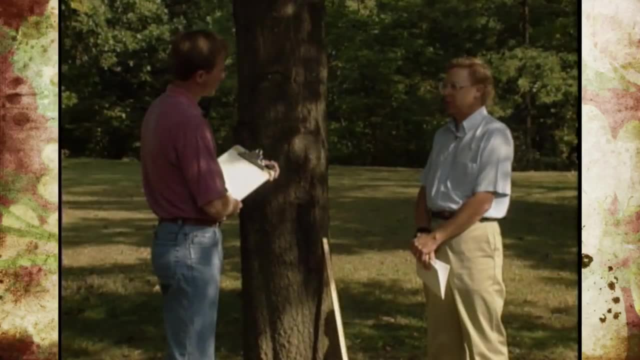 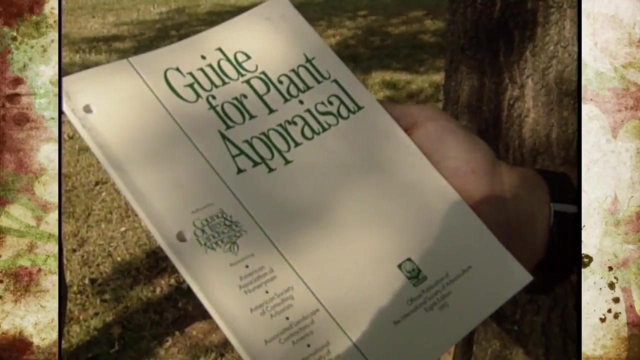 that group. Well, there's an organization called the Council of Landscape Plant Appraisers, and it is an umbrella organization of several different professional trade associations. The one that I'm most familiar with and that I am a member of is the International Society of Aboriculture, and that organization in fact prints and publishes a guidebook which 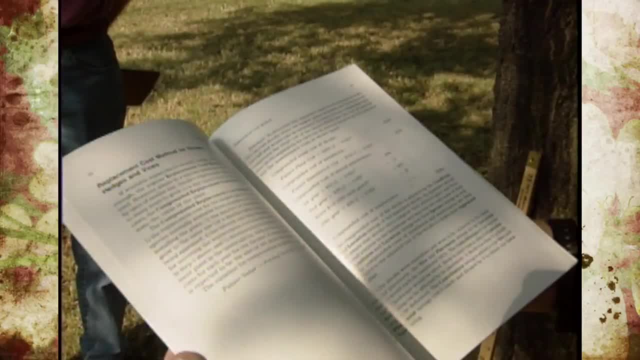 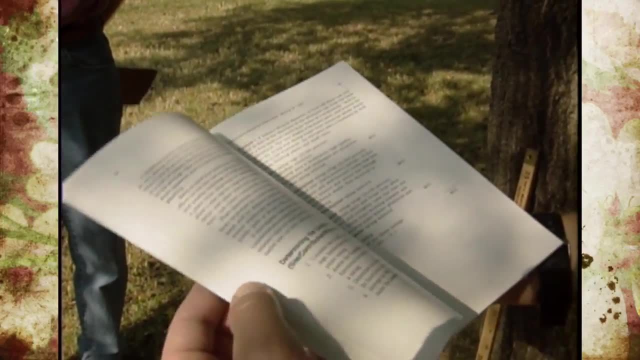 can be used by professional plant appraisers to help them through the process of the formula and understanding what it's about and how to determine a fair value of a tree. Okay, Tell us the new formula. I guess what did you say? that just came out in August. 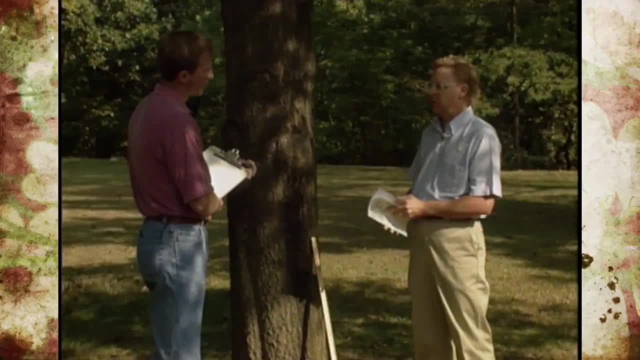 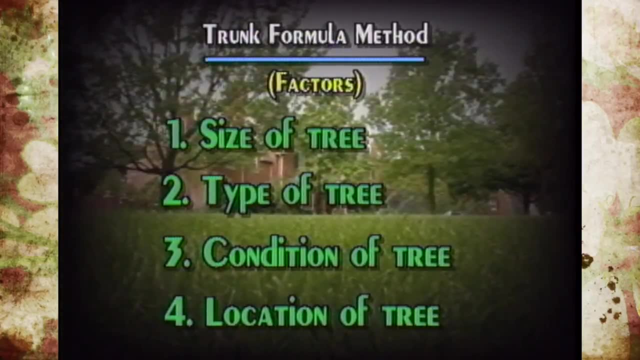 of this year. It was: yeah, they've been working on this for several years, and it was just recently, recently published, in August. Okay, What is the new formula then? Well, it's called a trunk formula method form, and it takes into consideration several factors. 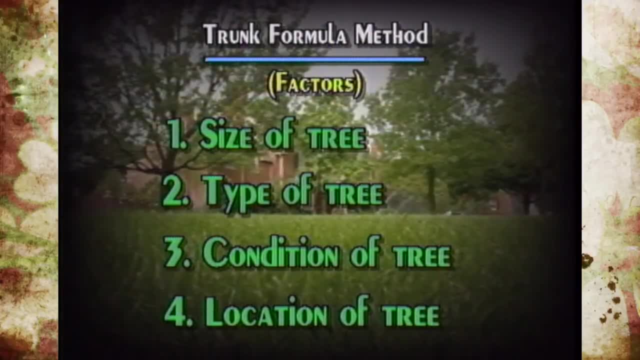 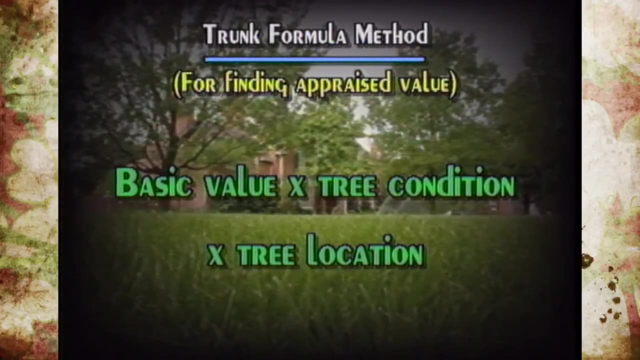 including the size of the tree, the type of tree, its condition and where it's located in the landscape. Okay, So the basic formula then, as I understand to get the appraised value, is the basic value times the condition, times the location. 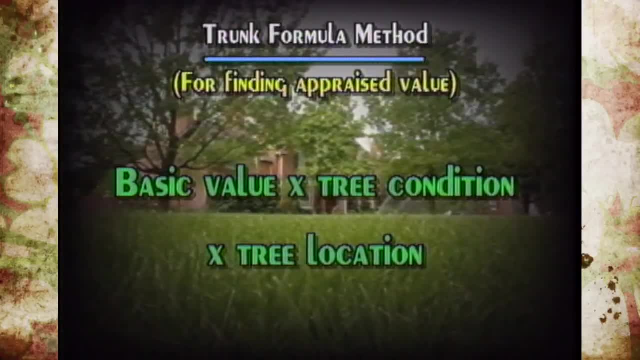 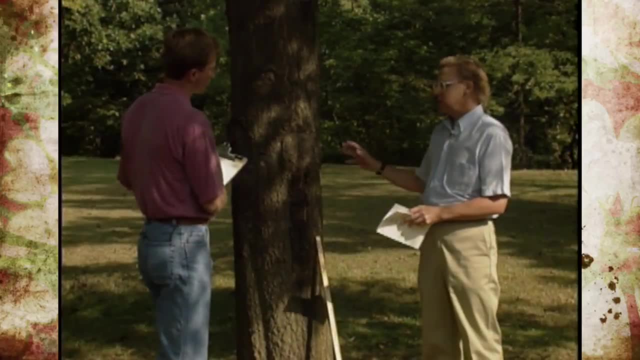 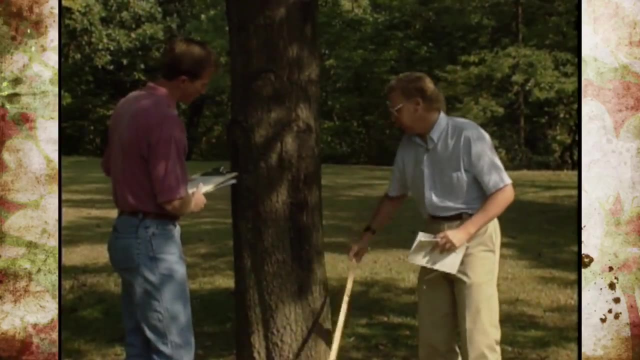 Now, that's a little bit different from what we've been used to Briefly tell us what things go into to determine the basic value then. Well, the basic value takes into comparison the area of the trunk of the casualty tree. This particular tree is. that's a 19-inch diameter tree. 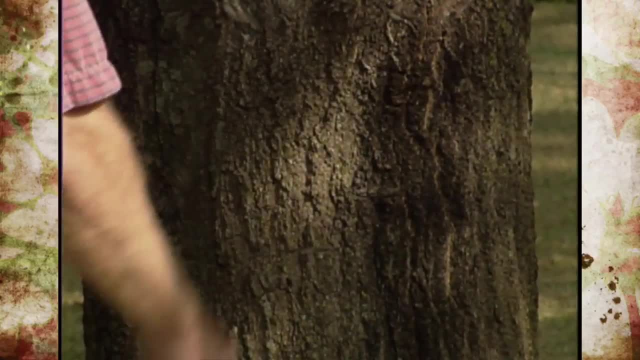 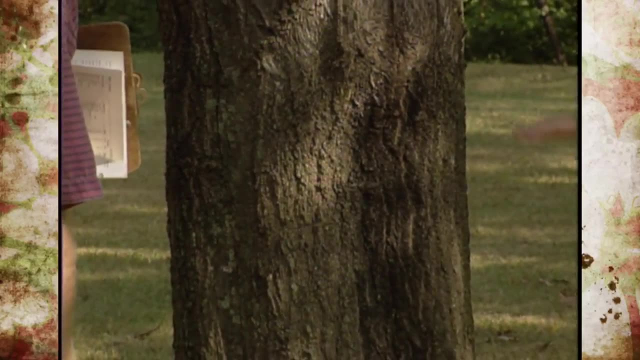 Okay, And where do you do you always have a standard location where you measure that too? Normally, we measure four and a half feet above the ground. Okay, Which is a which is a standard-look measuring point On this particular tree at four and. 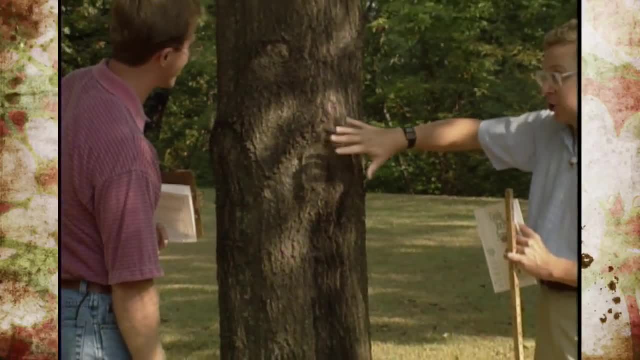 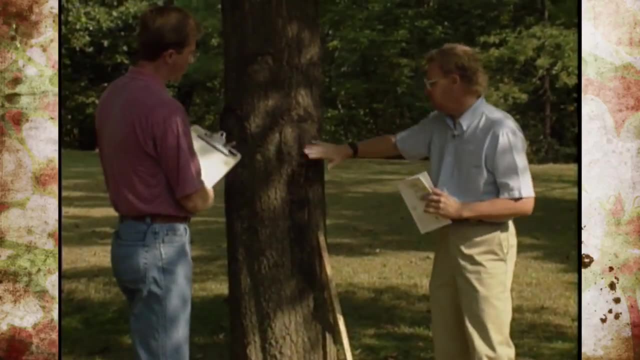 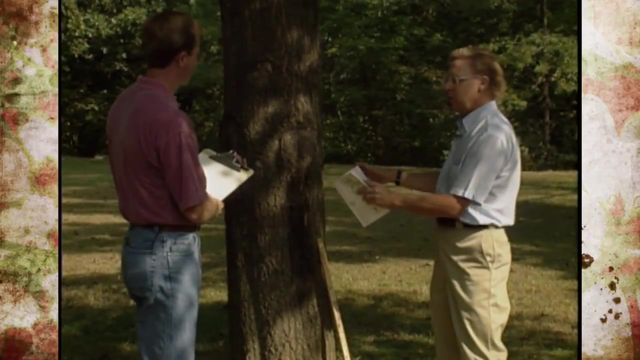 a half feet. there's an old branch here and this, this trunk is actually swollen, so we would get a false reading. Okay, So I measure just slightly below that point so that I would have a fair estimate of the diameter of this tree. We assume that the trunk diameter is circular and we convert. 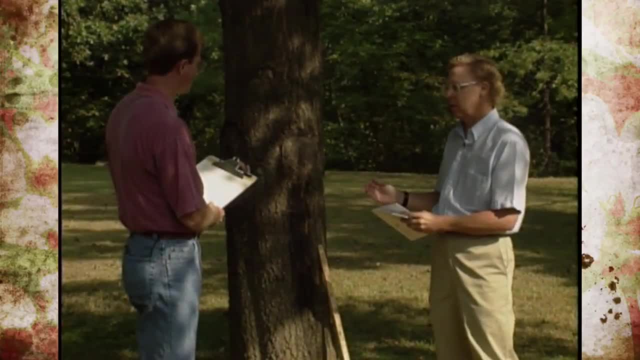 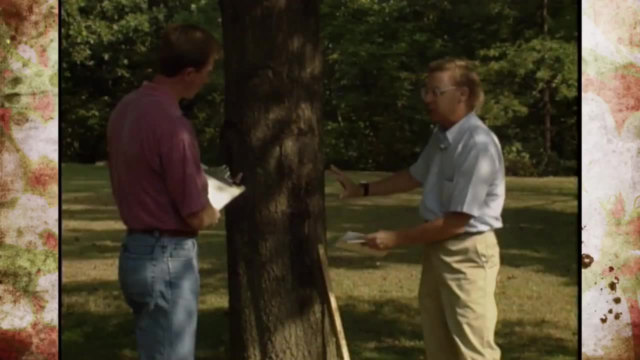 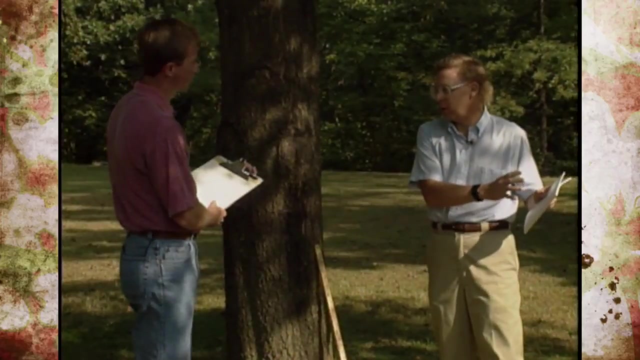 the diameter to square inches, and that's a straight mathematical calculation. Okay, And then what this new formula does is it compares the area of inches on this tree with the area of the largest commercially available comparable tree that we could purchase at a nursery. 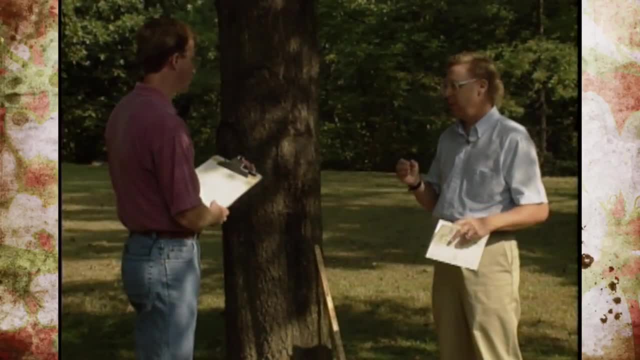 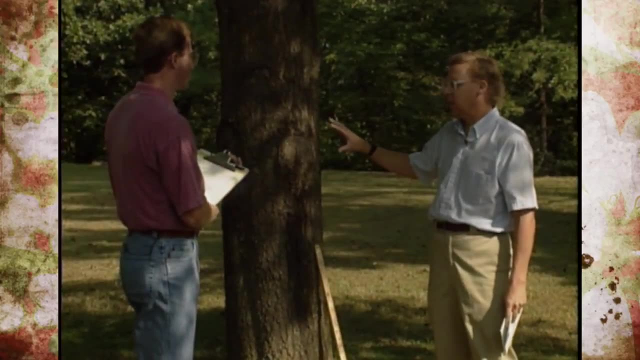 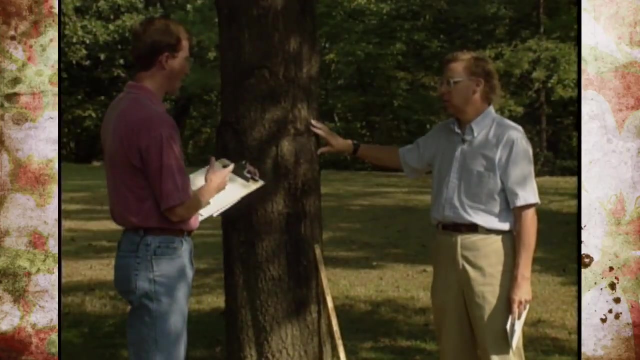 Okay, And then there's a difference in that size and there's a series of mathematical formulas that you would apply and steps to come up with a number that would give us a basic value for this particular tree. Okay, So the number that we used in these steps that we came up with was $9,923.68.. Now that 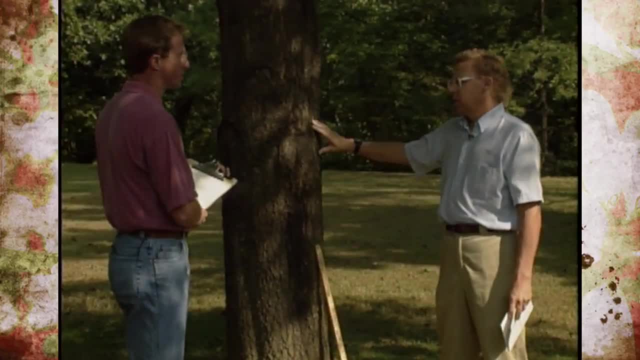 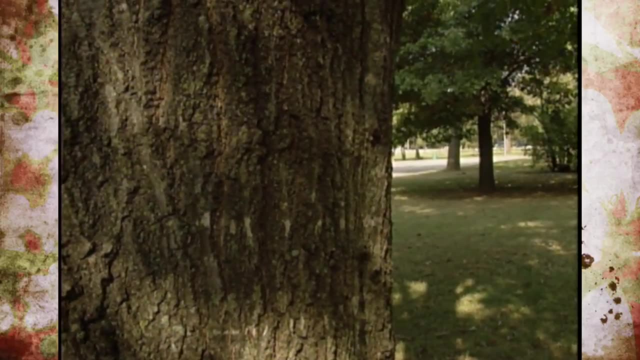 is multiplied by the condition. What are you looking at on the condition? There are lots of things that I look for when I'm looking at condition and trying to rate the condition of a tree. First of all, I look at the trunk of the tree. Is it sound? Does? 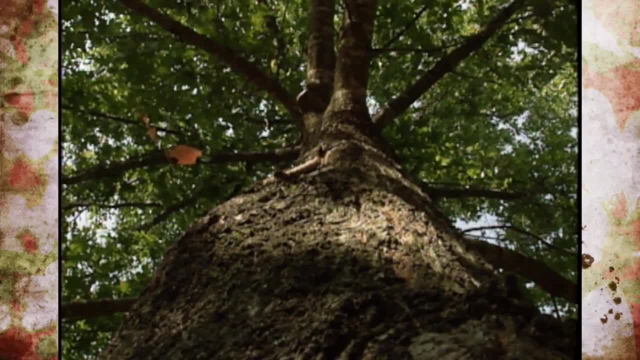 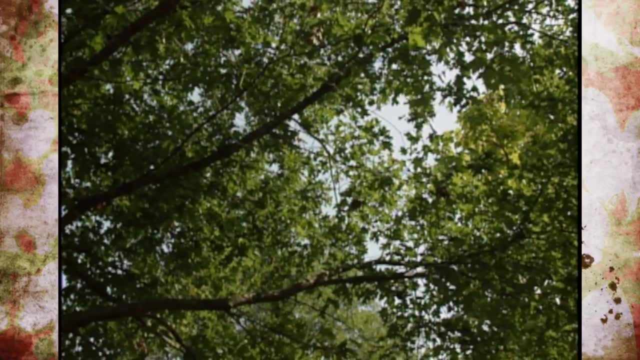 there appear to be any decay or old trunk wounds. I also look up into the tree and look at the branching structure. Is there deadwood up in there, or is there a lot of deadwood, or are most of the major branches in good shape? There don't appear to be any hazards. 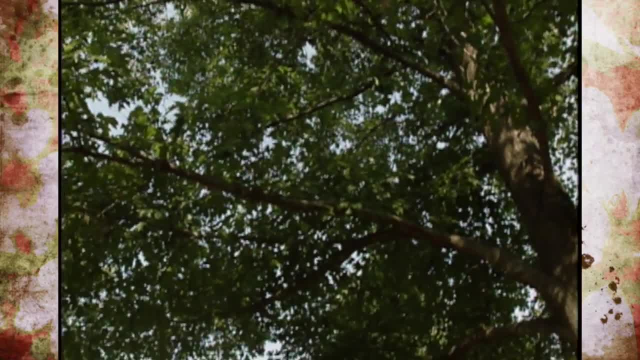 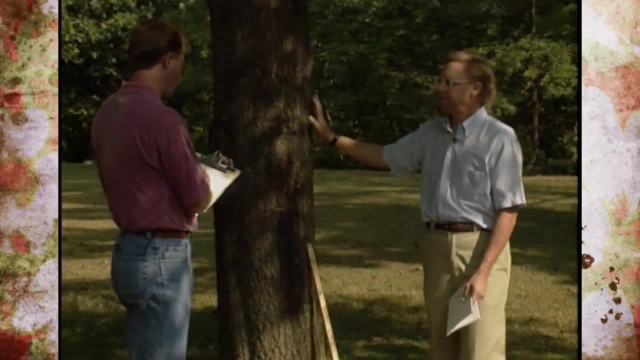 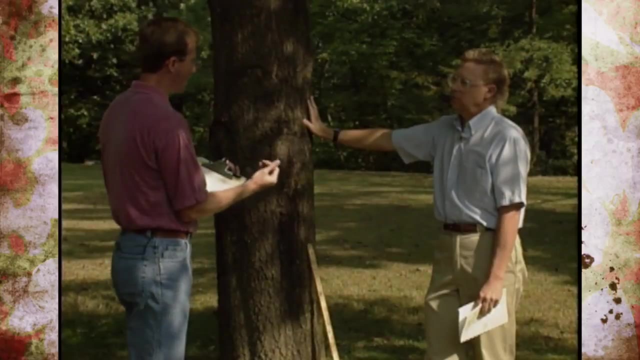 as far as snags or any other type of cracks or old storm damage or improper pruning practices in the past. Now, based on that point system that you give to, we came up with 80% or .80, and then that number multiplied by the other one is now multiplied by a number for the location and 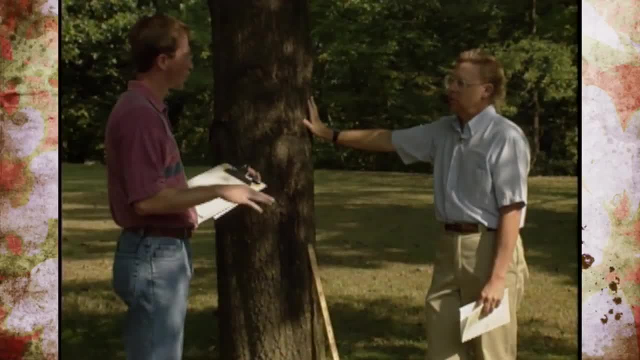 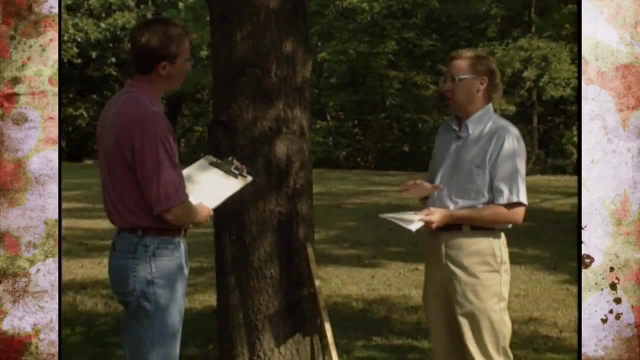 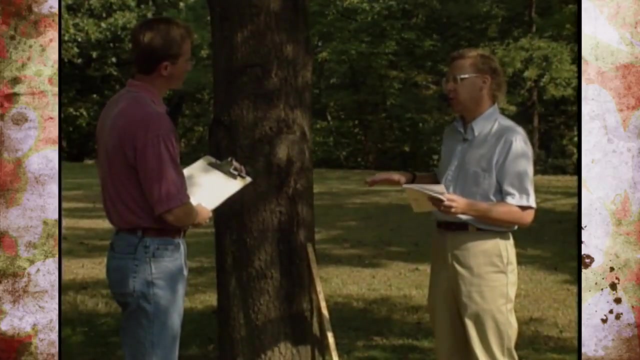 you gave it a .75.. Now, location in a park setting, like we're out here in Stillwater County. what are you looking at for location? Well, the location. they look at three factors in location. One is the site, which refers to the general site of the tree, whether it be not so much specifically in the yard or 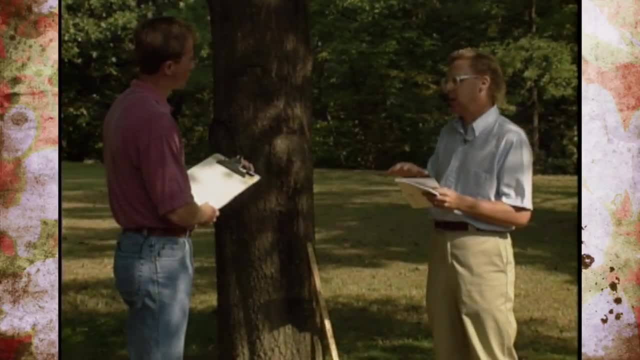 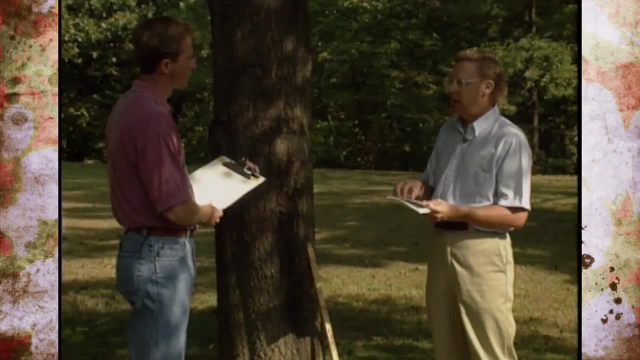 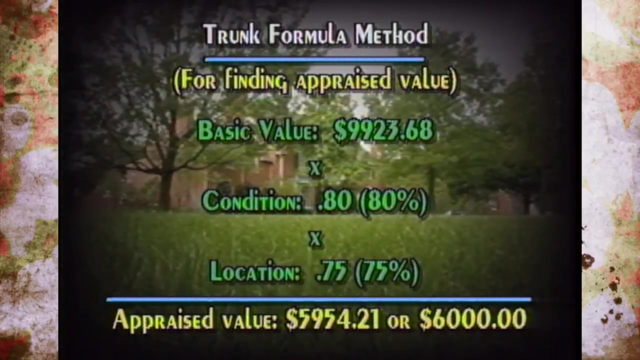 in the park, but perhaps a broader look at the site of where the tree is located, Also the contribution that the tree plays to that particular landscape, and then the placement of that tree within that particular site. Okay, And that number again was .75, so all of those numbers multiplied out we came up with 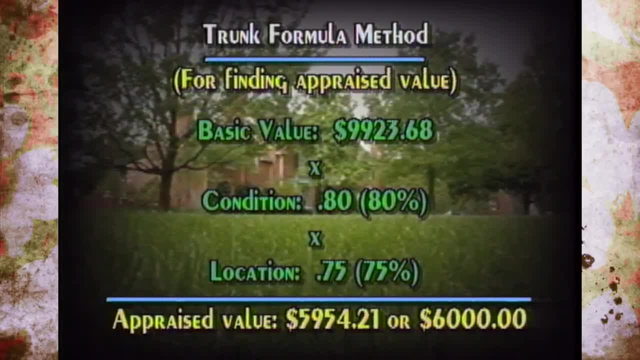 a praise value of this tree of $5,954.21, and in the directions I said to round it off. so we estimated about $6,000.. That's right Now. that's a little bit high in it compared to say, like the old formula. Why do you think? 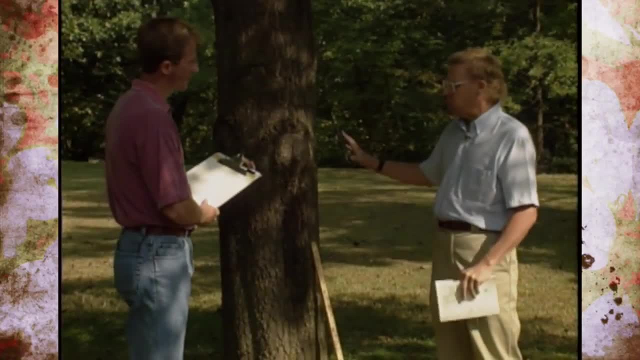 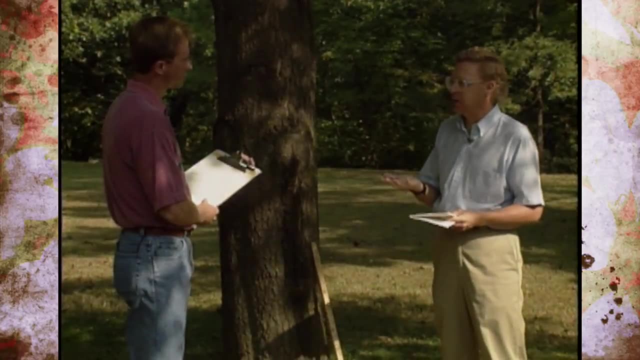 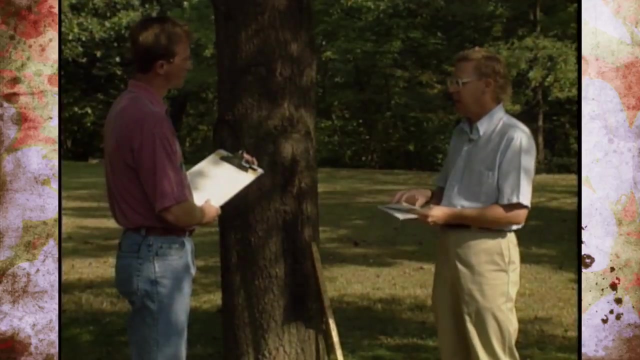 that would be Well. the old formula used a straight dollar value and that was adjusted periodically as inflation rates changed, Okay, And the cost of trees, purchasing trees, increased My as I understand it, the reason that there is a difference in value is that with the new formula, that's been changed, modified. 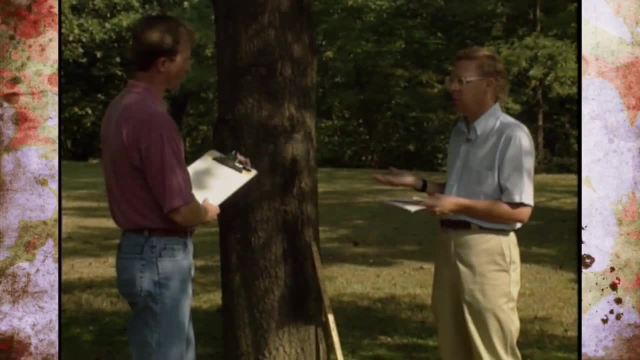 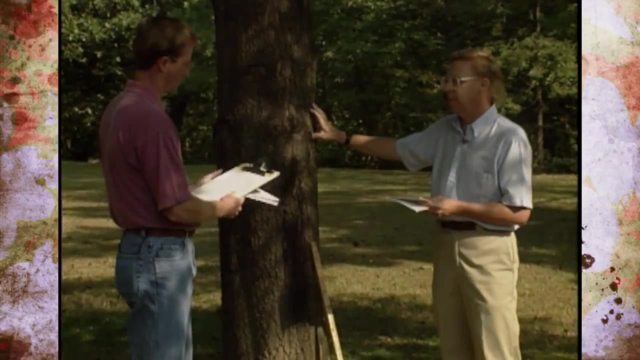 they have increased that basic dollar value up from the old value of $27, so there's probably a higher value built into that formula somewhere, which gives us which is the reason for the higher value, the appraisal value. Okay, All right. 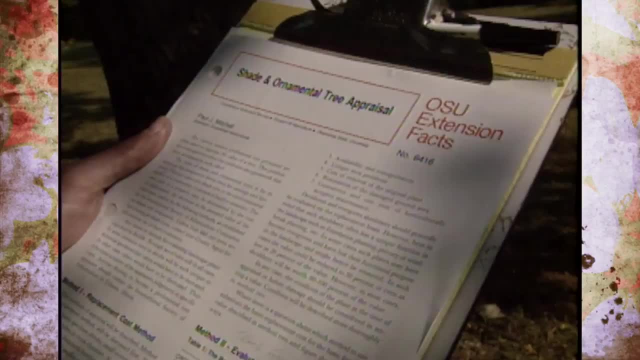 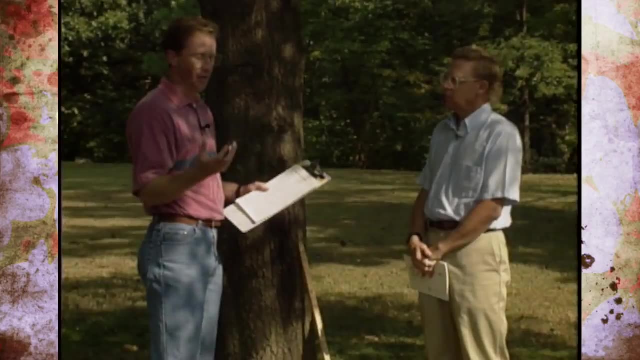 Well, of course you're familiar that we have a fact sheet, number 6416, that has the old formula in it and that's still going to be available until we can get it amended for the new changes. so a homeowner could go out and get this information from their 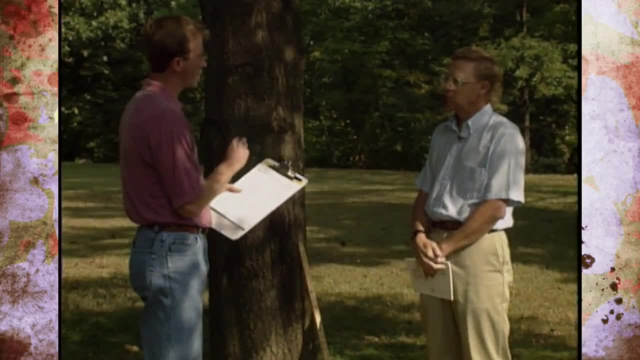 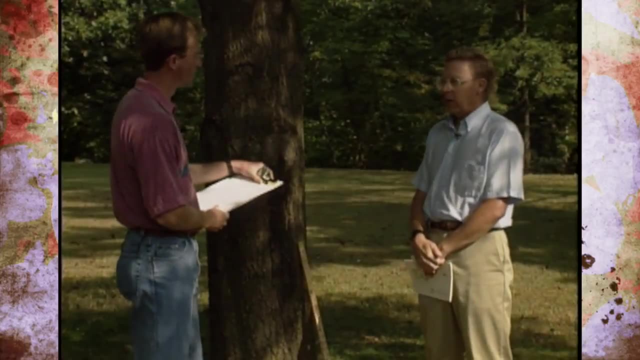 extension office, but I think what you're showing is that sometimes it is a little more complicated. How would an individual find an appraiser? What is the best way to go to find that information? Well, I would suggest that they can contact the state forestry office in Oklahoma City. 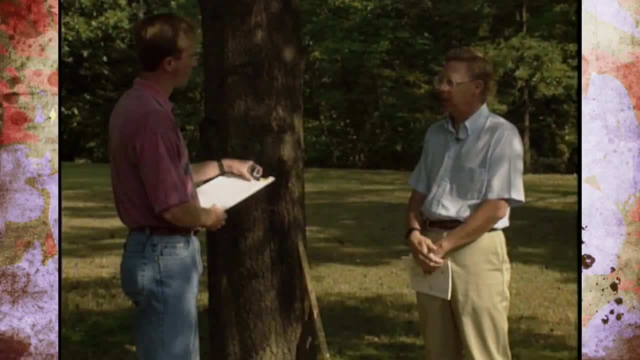 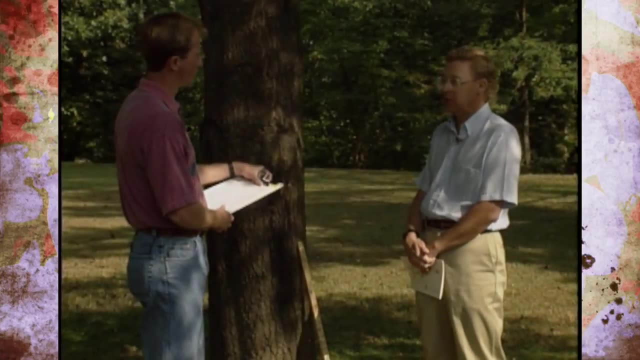 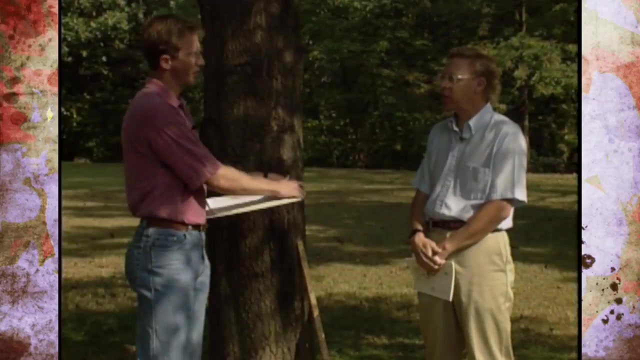 They have a list of Okay consultants in the state that they can mail out to homeowners. The county extension offices would probably have a list, perhaps the same list that the state has, but maybe even have a list that has local professionals that could perhaps do some kind of appraisal. 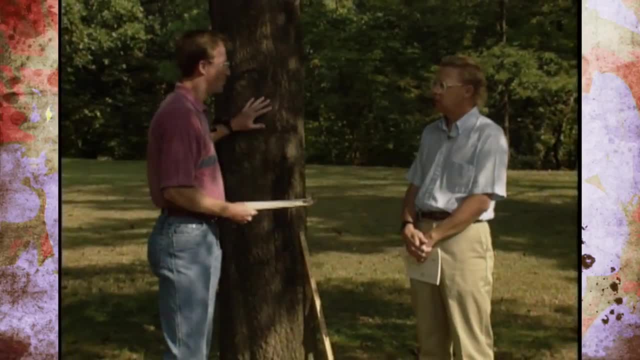 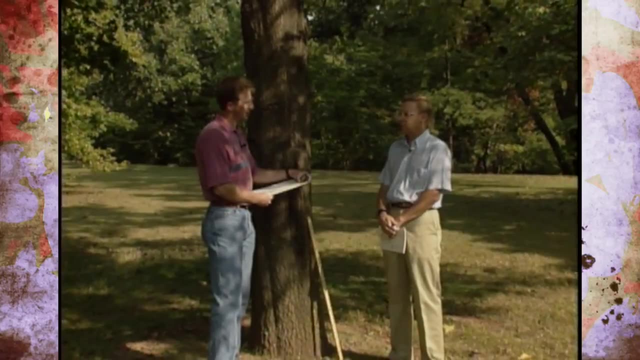 work. Well, Bob, the bottom line is: trees are a lot more valuable than we think they are. Would you like to comment on that? in many cases, Well, yeah, I think so, and many times when I have done appraisals and I give a number,